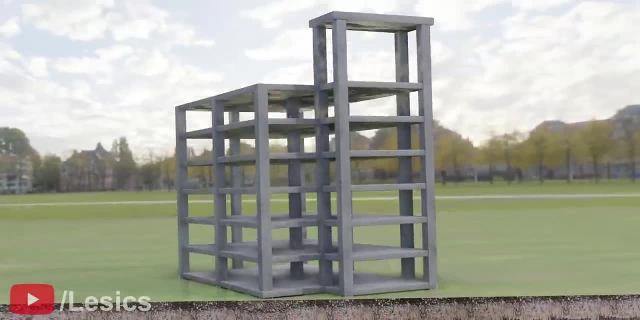 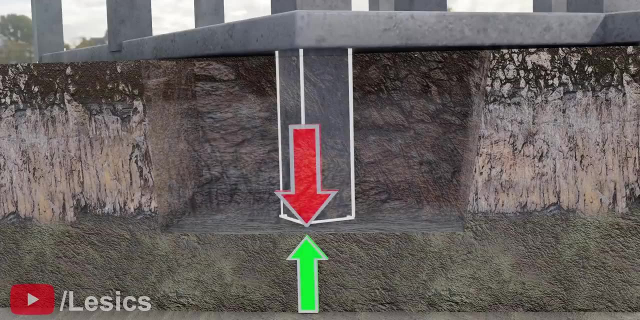 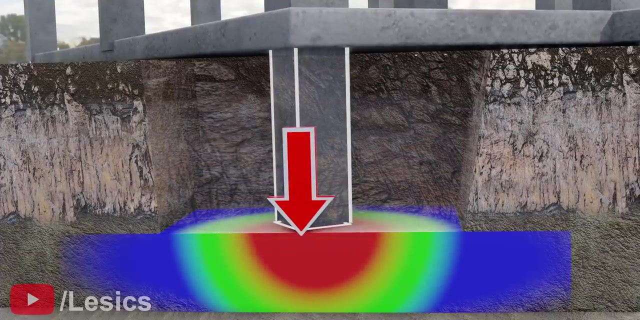 With this process, the soil should be able to bear the entire structural load quite easily. However, this concentrated load on the columns will cause excessive stress in the soil due to lesser contact area. If this stress exceeds the soil's bearing capacity, it will undergo the punching effect. 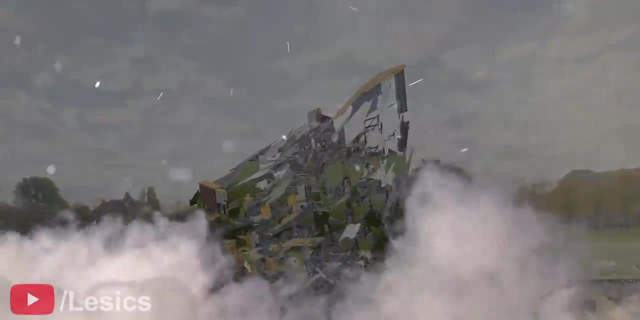 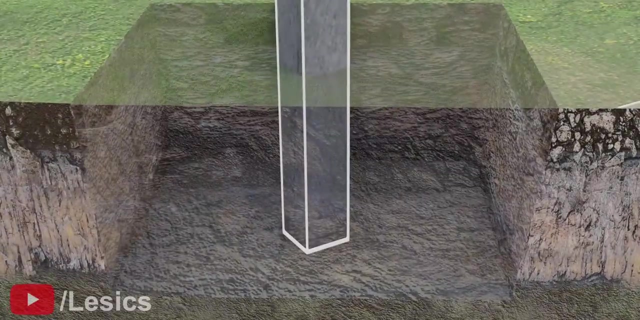 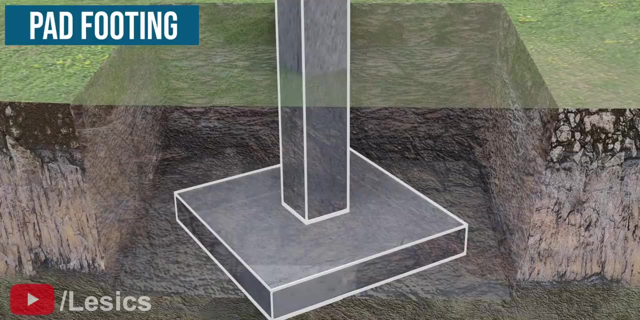 which leads to imbalance in your structure and eventually cracks or even failure of the whole building. To avoid these failures, you can increase the contact area between the soil and columns. Let's introduce a plate member that is the footing at the base of the column. 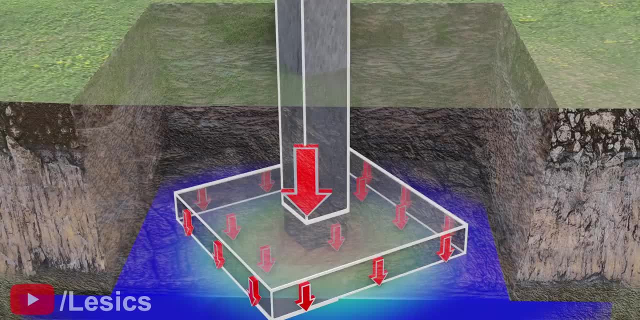 The load on the column will now be evenly distributed on the soil through plate members. This increased contact area reduces the stress on the soil and the building stands strong. The main job of a structural engineer in a footing design is to find out the area and 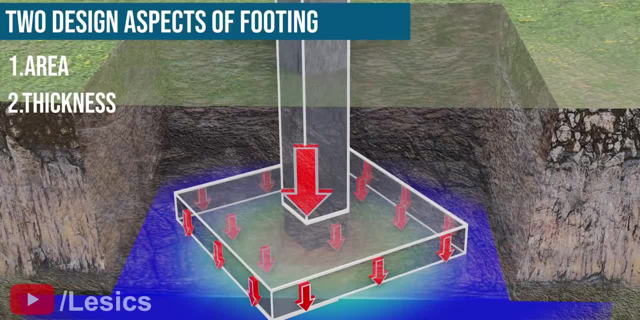 thickness of the footing. The main job of a structural engineer in a footing design is to find out the area and thickness of the footing. These two factors are determined by the contact area between the soil and the columns. The location of the contact area in the column is determined according to the bearing capacity. 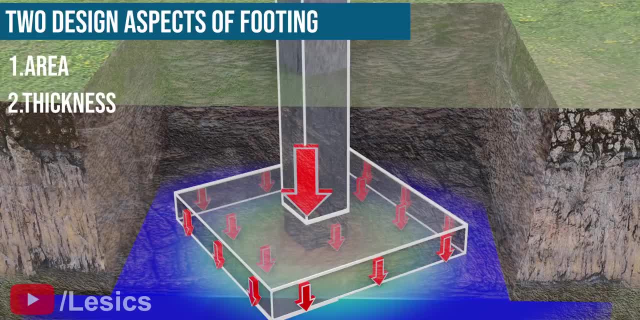 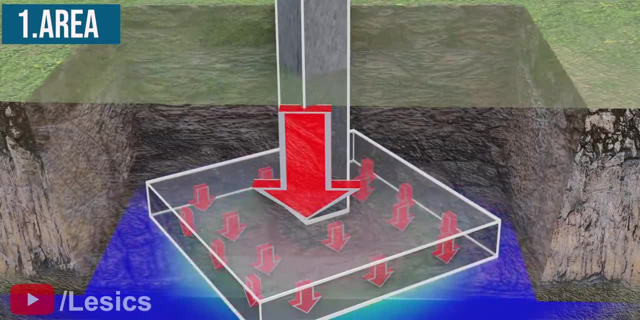 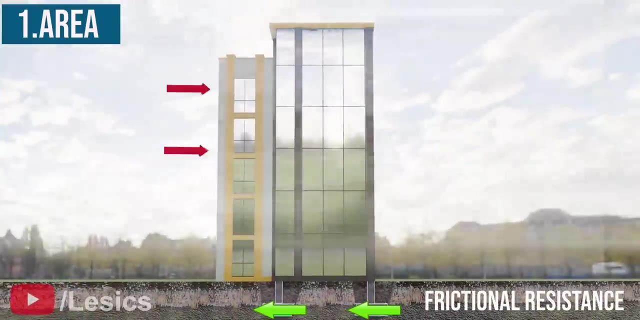 of the soil present on the site and weight of the building. We have already seen the importance of the footing area. More the weight of the building, wider should be the footing. Additionally, if this structure is subjected to lateral forces like winds, floods, etc. 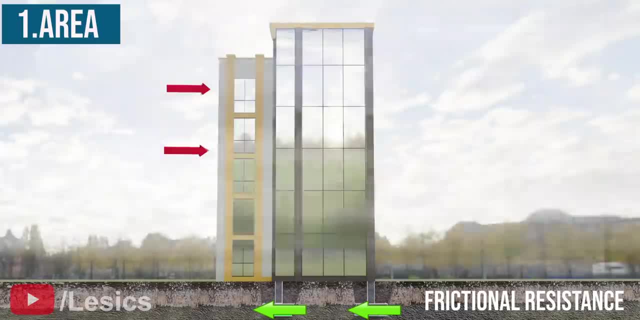 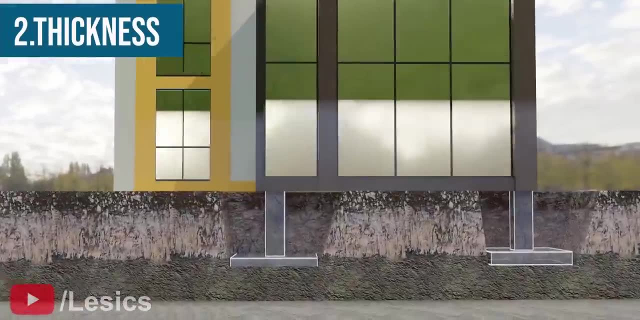 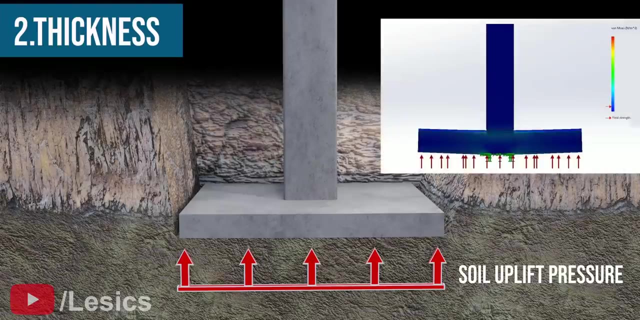 footings will help your building avoid sliding as a result of frictional resistance between the footing and the soil. 2. FOOTING design aspect: the thickness of the footing. The footing has to withstand pressure applied by the soil as well. If the footing's thickness is inadequate, the footing on either side of the 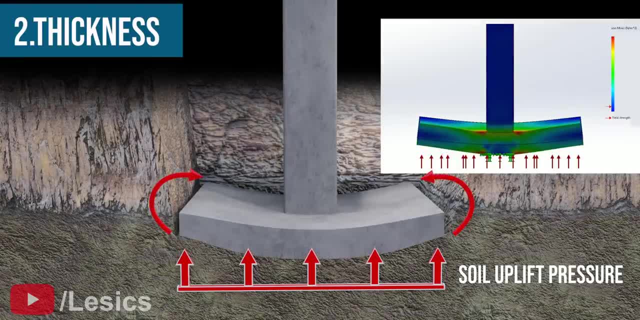 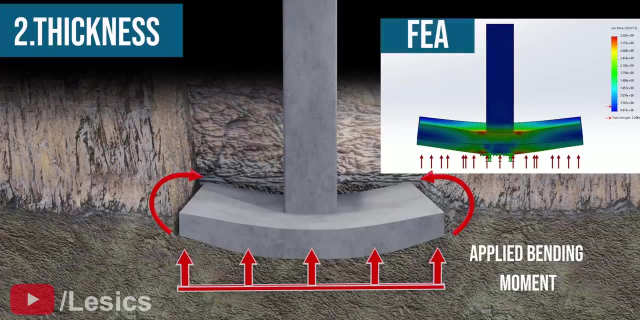 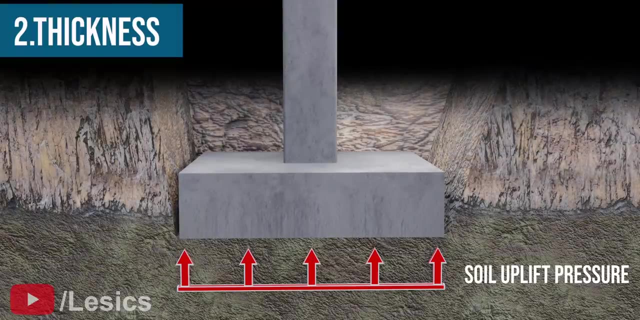 column will bend due to the soil applying uplift pressure on it. This effect is called applied bending moment. You can see this effect in this FEA result here, To prevent this result, the thickness of the plate is increased. There you go. We have designed a stronger and safer footing for 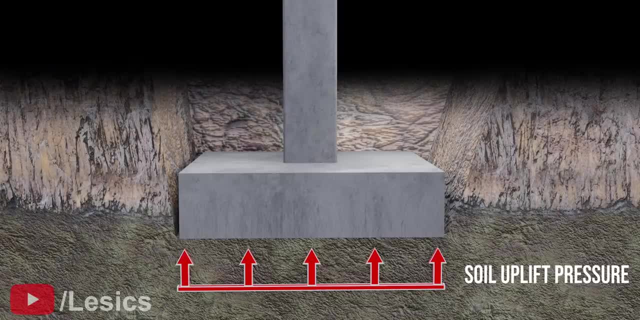 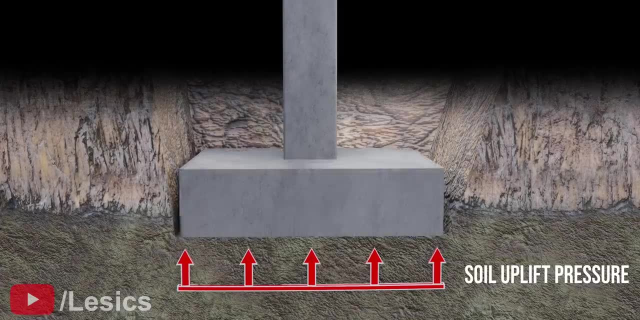 our building. This type of pad or isolated footing is employed to support lightweight houses that rest on soil with medium strength. This design can be further optimized economically. If you observe the pressure applied from the soil on this area, it is uniform, However applied bending.